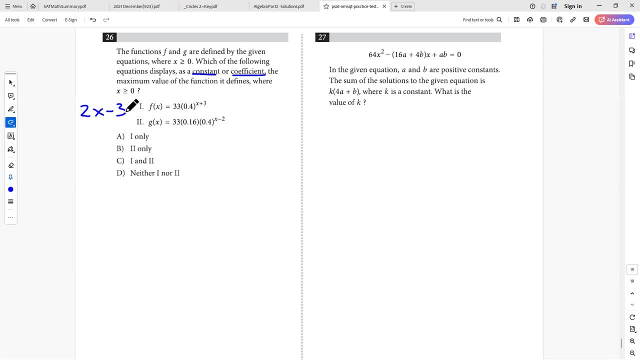 change. coefficient is a number that is multiplied by the variable. that will be the two. here will be a coefficient. Okay, we have to deal with the maximum value of the function. Okay, what type of functions are these? We have the variable exponents. So these are exponential functions, The value that it's inside the parentheses here. 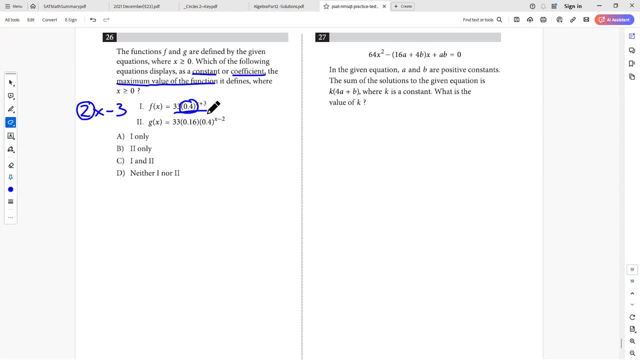 is 0.4.. So if I multiply somewhere by 0.4, it will decrease. If I multiply that result by another 0.4, that will decrease. So these are exponential decay functions. here They will decrease as x increases. So the maximum value would be the least value of x, the value of the exponent that we 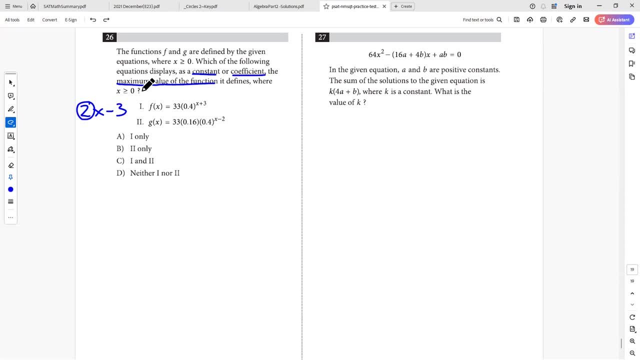 have. So the least value of x here would be- since x is greater than or equal to 0, would be 0. So the maximum value of the function will occur when x is 0. So let's figure out what the maximum. 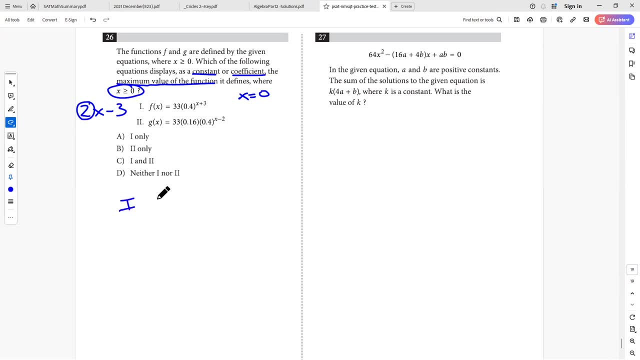 value was of each one. So the first one is going to be 33 times 0.. 0.4 to 0, plus 3 power, which is 33 times 0.4 to the third power, And it gives you 2.112.. 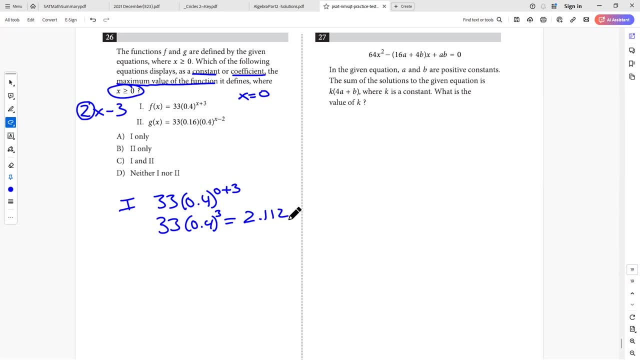 All right. so does that number- 2.112, appear as a constant or coefficient in that function? You have to say that's no, because we see 33,, we see a 0.4, and we see a 3. So there's no 2.112.. 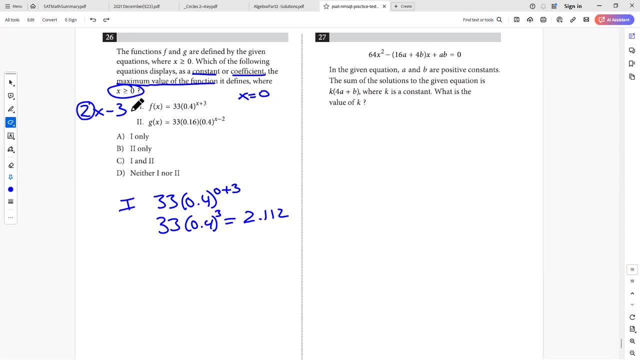 All right, so definitely not that one. Let's try it in the second one. So it's going to be 33 times 0.16 times 0.4.. Again, 0 will give us the highest value there. so 0 minus 2, or just a negative second power, And we'll apply that out. 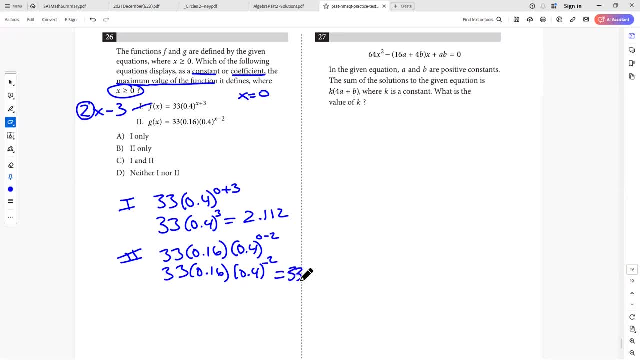 Thank you. And it gives us 33.. So does 33 appear as a constant or coefficient in that function? And it does, right there, Okay, so 2 is true, And that's the only one that's true. so the answer is b. Now the second one. we have 64x squared, minus the quantity 16a, plus 4bx. 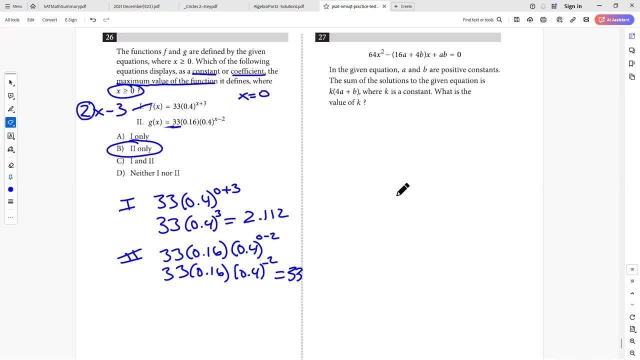 plus ab equals 0.. In a given equation, a and b are positive constants. the sum of the solutions to the given equation is k times the quantity 4a plus b. where k is a constant, What is the value of k? All right, so one of the key things to do on the SAT. 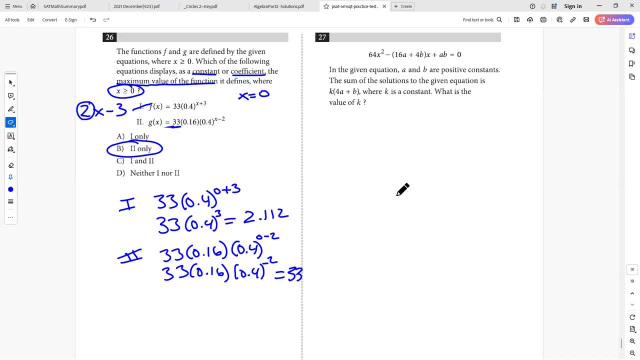 is to be able to identify the type of equation it is and identify any kind of formulas we need to do to help solve it. So we have x squared, the highest exponent is a 2. So it's going to be quadratic or parabola And we're dealing with the formula. and we're dealing with the formula. 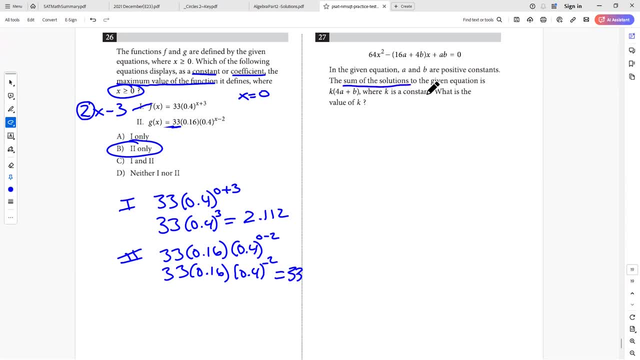 and we're dealing with the sum of the solutions of a parabola. Okay, that's equal to negative b over a. We're referring to ax squared plus bx plus c equals 0.. Okay, so we just need to use that formula and get it into this form: k times the quantity 4a plus b. Now don't let the a and b's 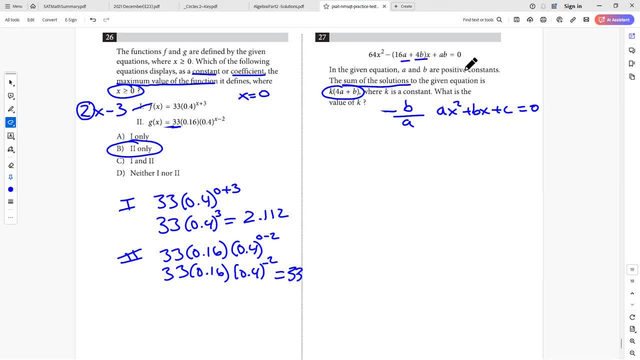 that appear here confuse you, Okay, because the a we're referring to this is the coefficient of the x squared, So that's the 64 is a. The b is a coefficient of the x term, So that's this negative quantity of 16a plus 4b. 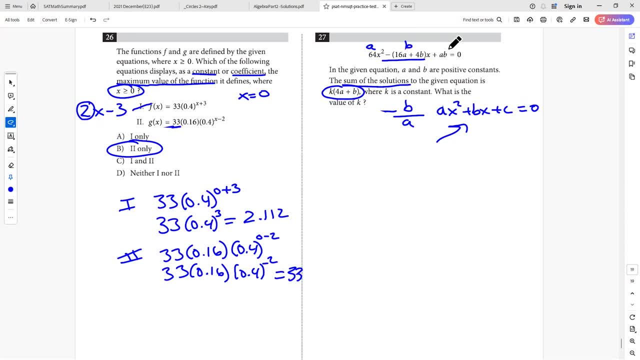 So that's our b value, And then the ab here. the constant value here is going to be c. Okay, so we need negative b over a. So it's going to be negative. And then we have negative 16a plus 4b over our a value, 64.. 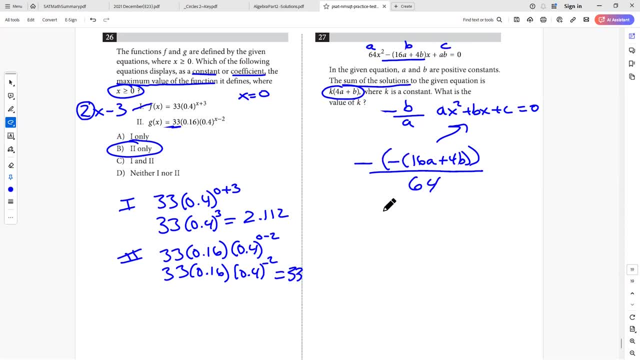 And the two negatives will cancel out giving you a positive. So we just have 16a plus 4b on top over 64.. Okay, and we need 4a plus b. Notice, here we can factor out a, 4 on top. 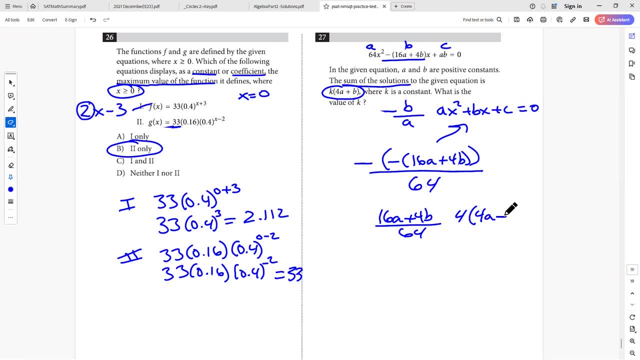 Okay, so it's 4a plus b. Okay, I'm going to rewrite that as 4 over 64 times 4a plus b. If I want to reduce it, you don't have to. That's 1 over 16.. Okay, so now we have it in our form that we want k times the quantity 4a plus b. 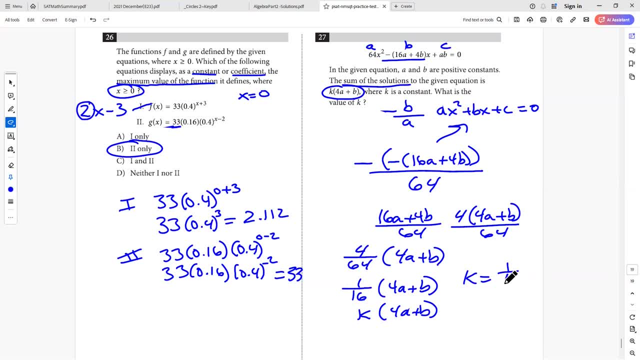 So k would equal 1 over 16.. Okay, so again the quadratic went to sum of the solutions. Sum of the solutions is negative: b over a. If they wanted the product of the solutions that would have been c over a. 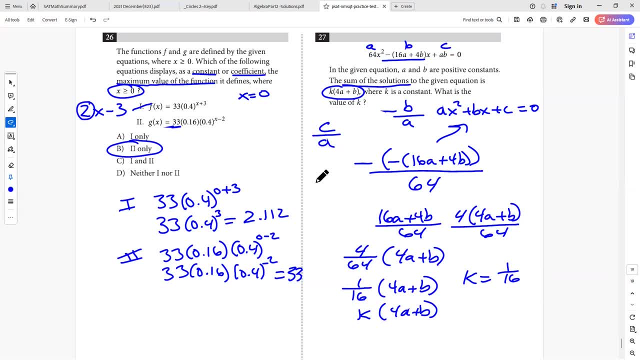 Okay, so again, identify the problem, identify the formulas that you need to use and solve that problem. All right, I hope this video helped you understand Some things about the digital SAT. If you enjoyed this video, please like it and share and leave a comment. All right thanks. 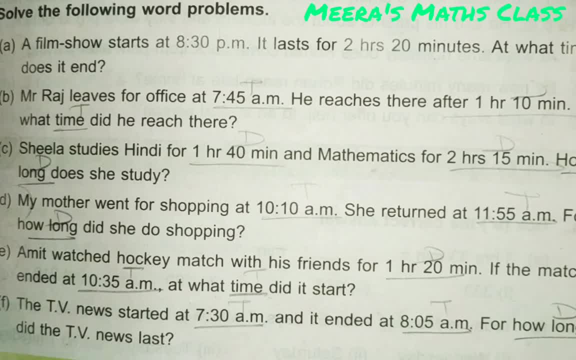 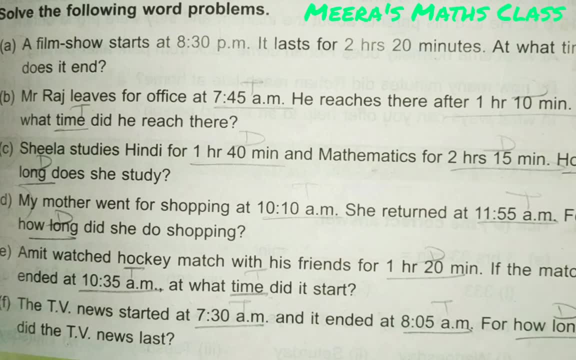 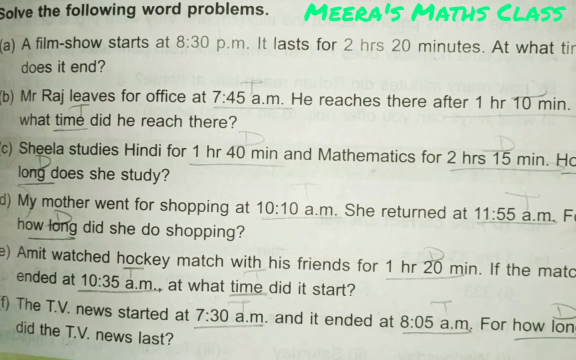 Hey, welcome to Meera's math class. Yes, now, my dear children, we are going to see the word problems of time chapter. Now, as I told you, there are two type of times which I say: One is exact time and the other is duration. 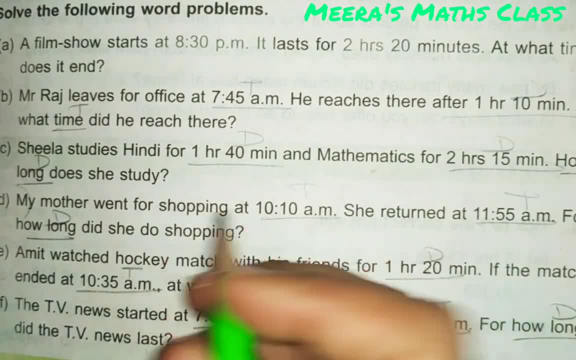 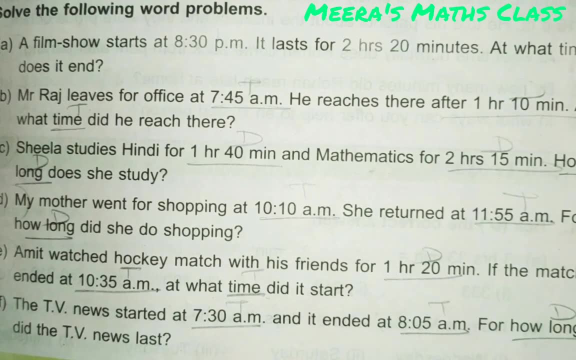 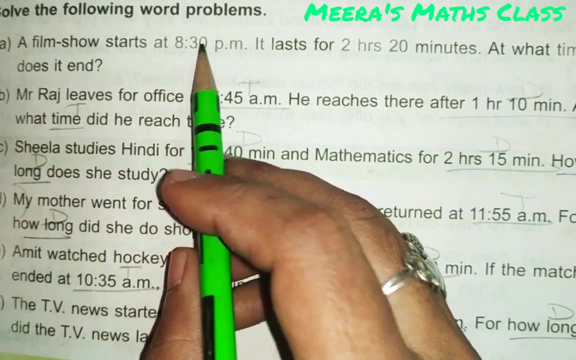 Now. first you have to read the word problems and you have to write which one is the time and which one is the duration. First thing you are going to do that. Let's see the first example. A film show starts at 8.30 pm. 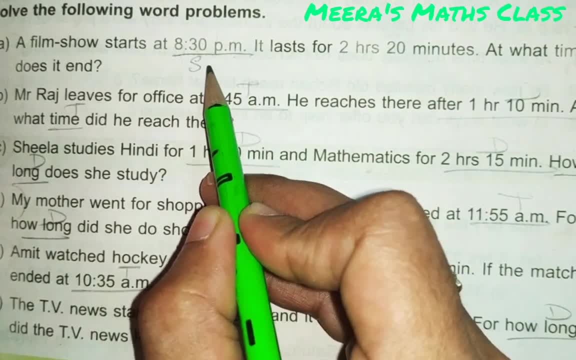 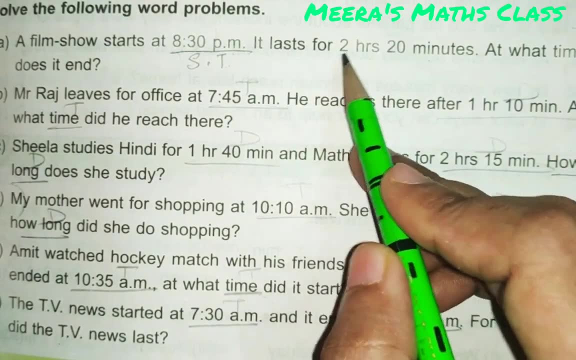 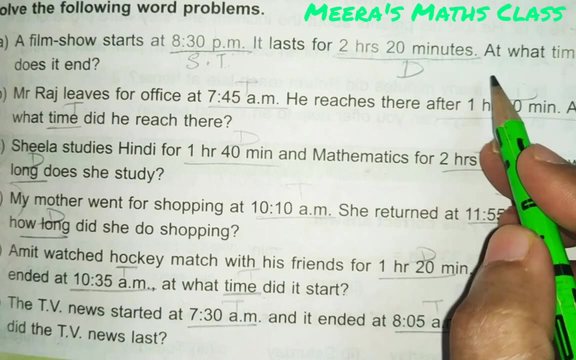 So this is the starting time. You can write even that this is starting time. ST for shortcut to understand. It lasts for 10.. 2 hours, 20 minutes. Now underline this What it is. This is duration. Let's write it as D.